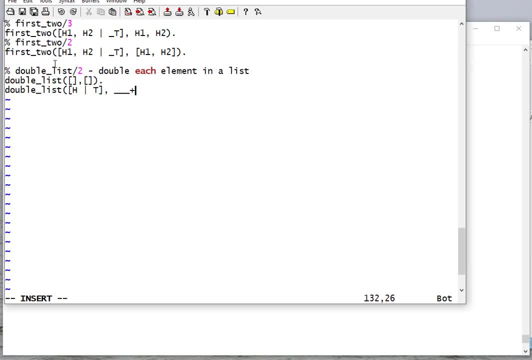 but I'm going to leave this blank for now and we'll come back to what we're going to put there. The first thing is that I need to double the head, so I'll do that with some math. I'll say: h2 is h times 2.. 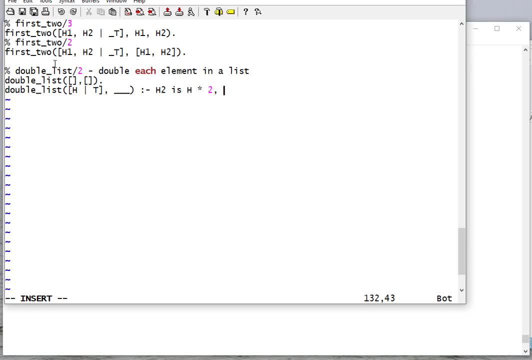 And then I'm also going to need to double everything in the tail. so that's a recursive call And that'll give me- I'll call it t2, so that everything is doubled. So now the question is: what is this result? 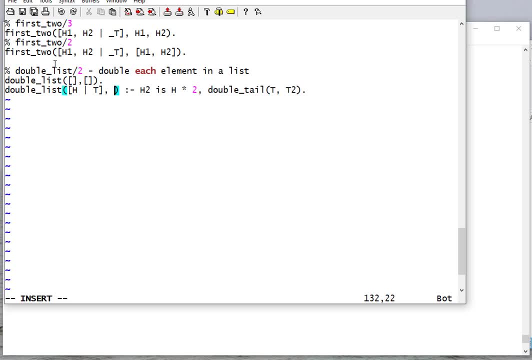 Well, the result is the head put in front, or head 2 put in front of tail 2.. So h2, which is 2 times the original head, And the tail is going to be the tail, with everything doubled. So this completes my rule. 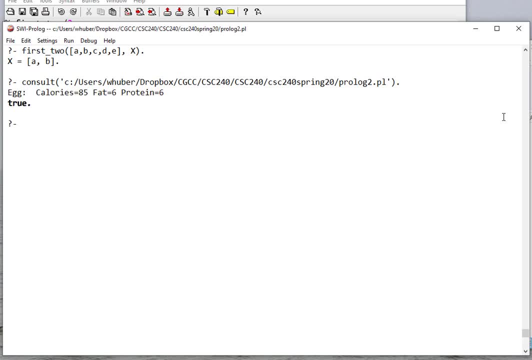 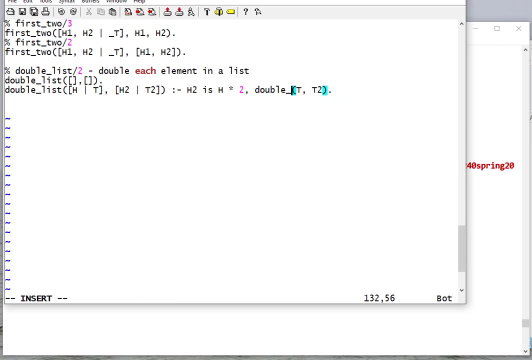 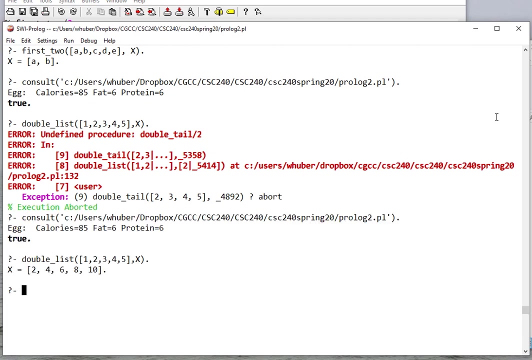 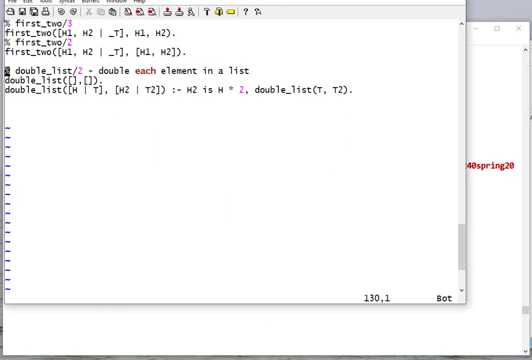 So let's consult. Did I call it double tail? I did So. what happens when you talk and type at the same time? So now, when I double the list, you can see every element is doubled. I could also, instead of doubling the list, 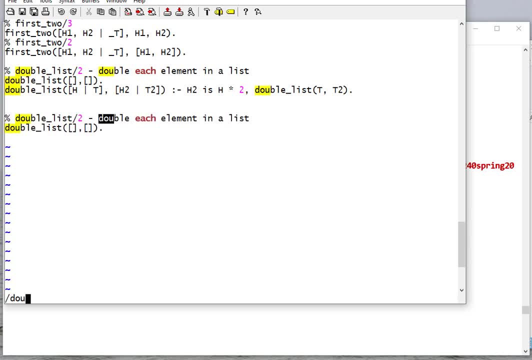 I can duplicate the list elements. I can duplicate the list elements. So here in my recursive case I'm going to have a head and a tail And I'll leave the result for a moment. I don't need to do anything with the head yet, but I do need to duplicate the list elements in the tail. 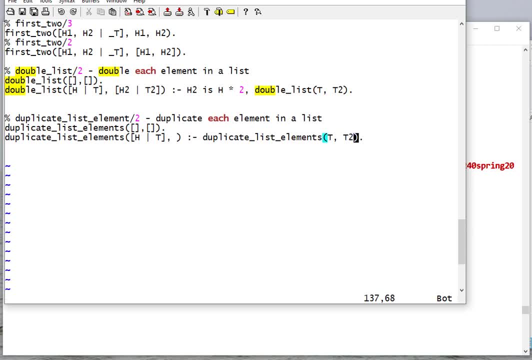 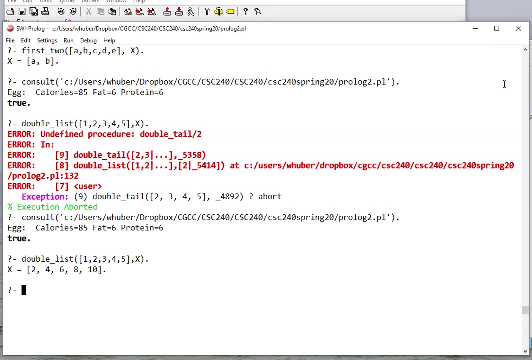 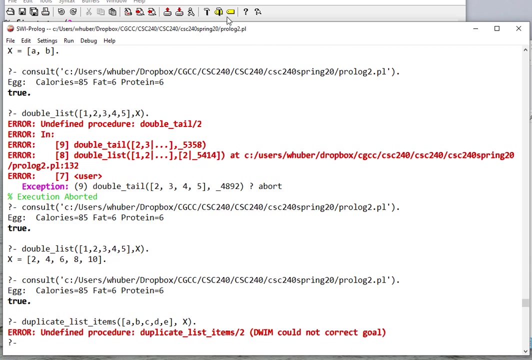 And I'm going to do that, And then my result is going to be two copies of the head element with the tail after I duplicate everything. So let's consult, Let's consult. Did I say elements, Elements, So I'll duplicate list elements. 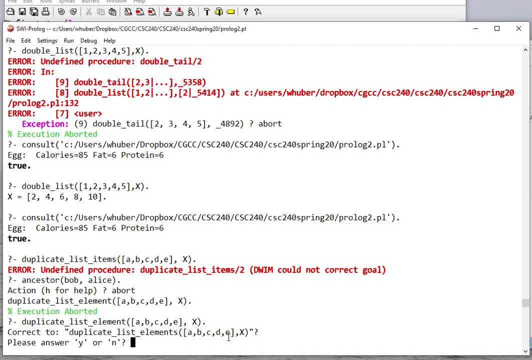 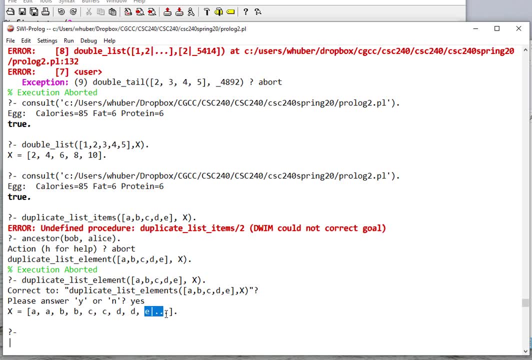 And something bad happened. Duplicate list elements: Yes, So I'll answer yes. And so there you see: A, A, B, B, C, C, D, D, E, E, And whenever you see this, it just means that the list was too long and it gave up trying to display it. 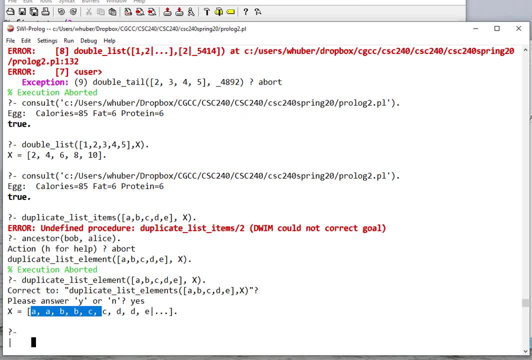 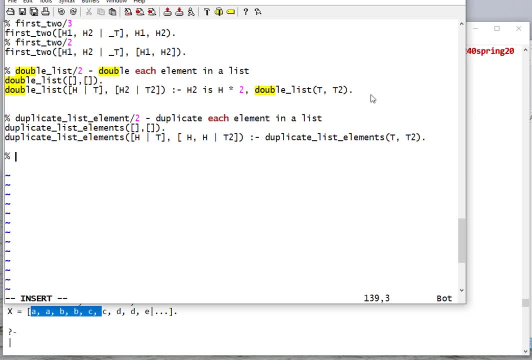 So don't be alarmed if you see this. As long as your list starts out looking good, then you'll be okay. So next to we'll check that two elements appear next to each other in a list. My base case is not going to be an empty list here. 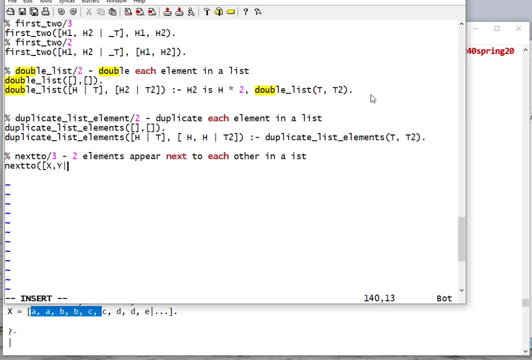 If I have an X and a Y, they need to be empty. They need to appear next to each other in the list somewhere. I don't care what the tail is in that case, because now X and Y do appear next to each other. 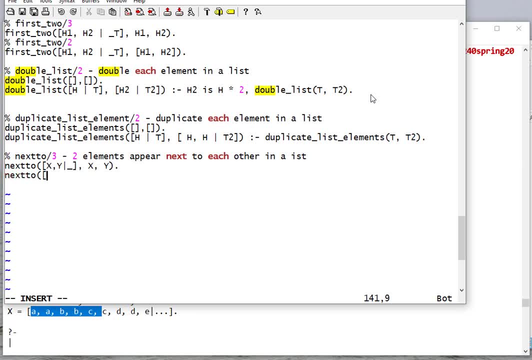 Otherwise, what I'm going to do is I'm going to get rid of the head And I'm going to look to see if X and Y are next to each other in the tail. So I'm not actually returning a list here, I'm just returning true or false. 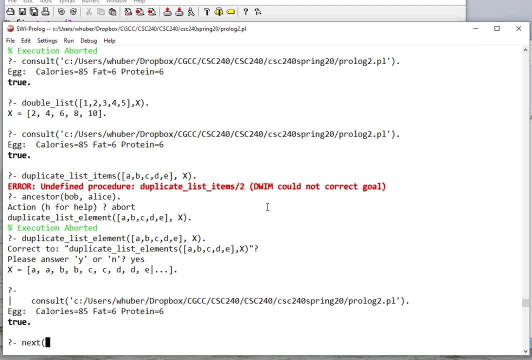 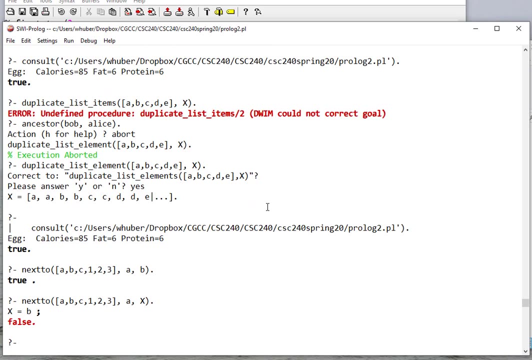 So we consult And now let's send the list: A, B, C, 1,, 2,, 3, our A and B together. That's true, Okay, so what is A next to B and nothing else? So what if we say we'll say AX here? 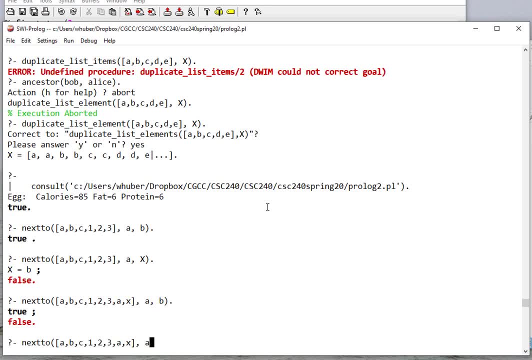 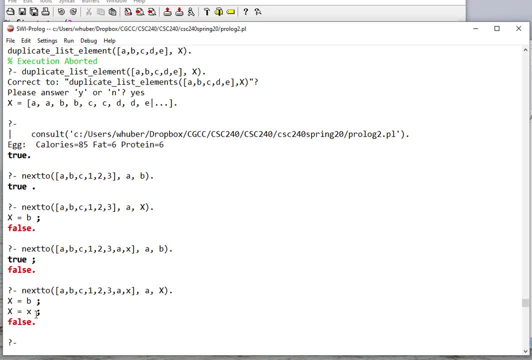 So that's true And I didn't give these variables. So let's say A is next to X, B, X and false. So it actually, when I rejected it, it kept looking for something else that that atom could be next to. 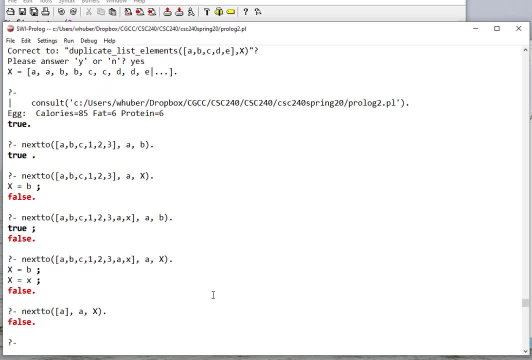 If I give it a list that's too short. it doesn't match that base case, The base case. we have to have at least two elements, And those would be the two elements that we are looking for next to each other. Let's write some methods that do some summing. 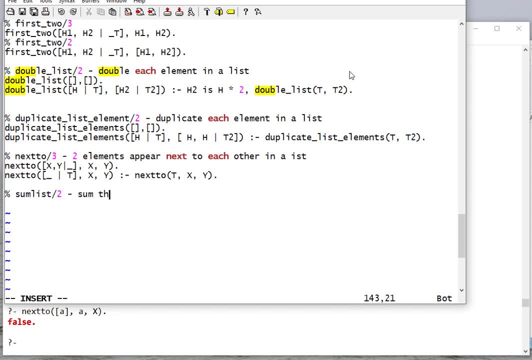 Okay, So this is going to. this rule is going to sum the elements of a list. So the sum of an empty list is our base case And that sum is going to be zero. Then, to sum the list with some head and tail, we're going to get a sum. 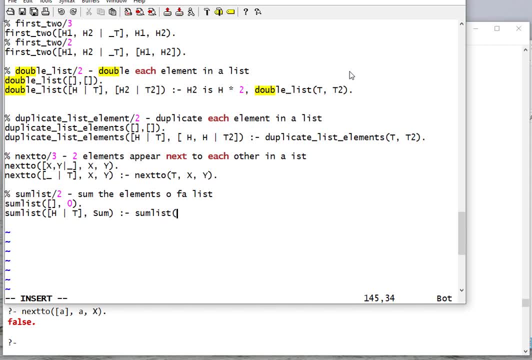 But to get that sum, first we have to sum the tail, And that's going to give us the sum of the tail, Then the sum. the final sum that we're going to return is sum T plus H. I can also write a rule that sums the first X elements of a list. 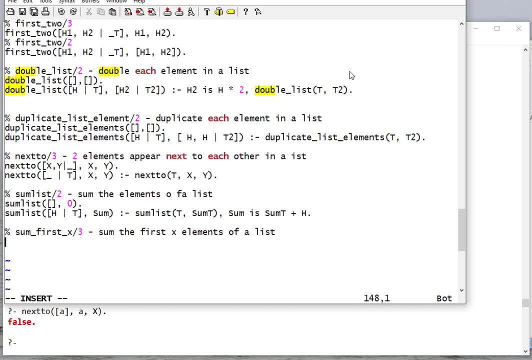 And that's actually going to take three parameters, because I need to pass in how many. I want them to do. So sum first X, And in here I don't care what the list is, If there's, I'm summing the first zero. that result is zero. 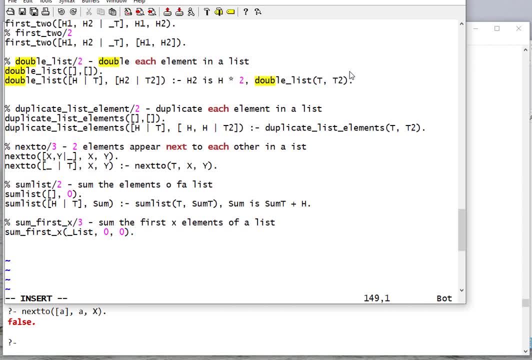 So it's almost like that's the base case: where there's an empty list, There's nothing left. to sum here A recursive case. I'm going to have some list And again I don't have to check If that it's a list, if I give it this list syntax. 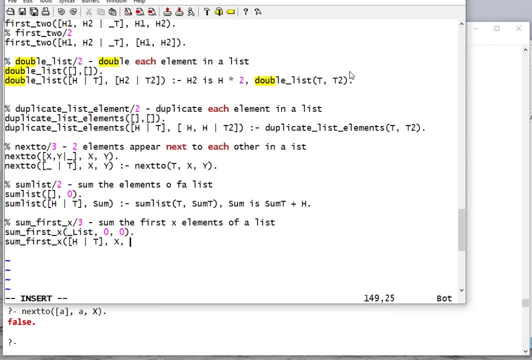 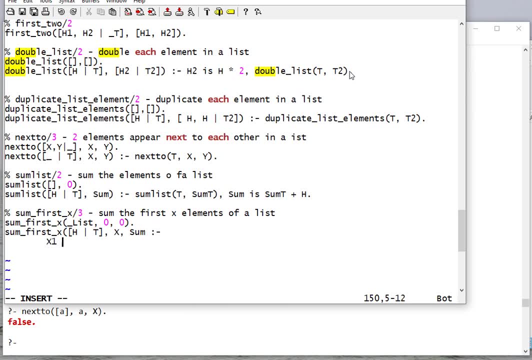 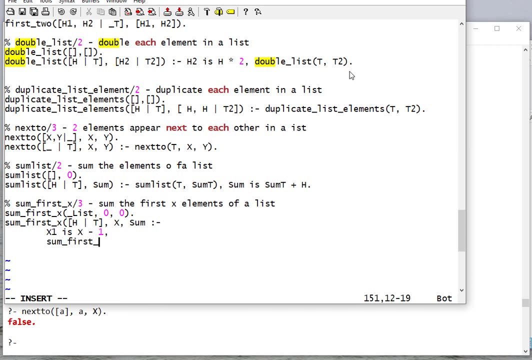 the only thing that would match here is a list, The first X elements and the sum. So now I'm going to say X one is X minus one And that's going to allow me to find the sum of the first X minus one elements of the tail. 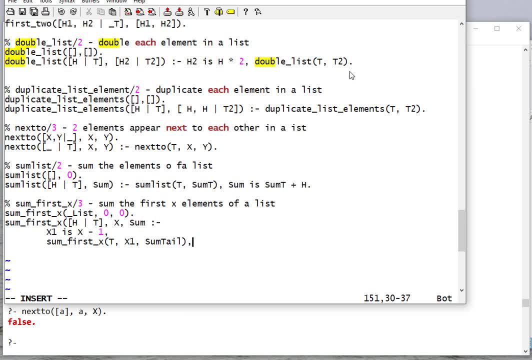 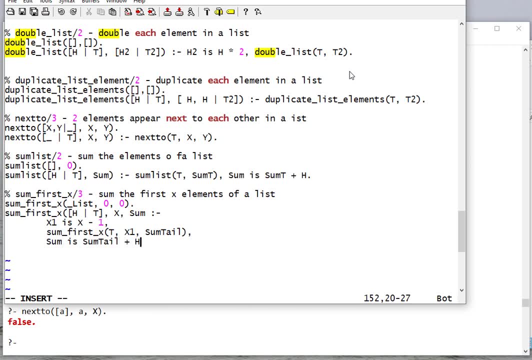 And that gives me the tail that I get from the list, The sum that I get from the tail, And then the final sum is going to be sum tail plus H. So notice here I'm subtracting one from X each time as I go through the tail. 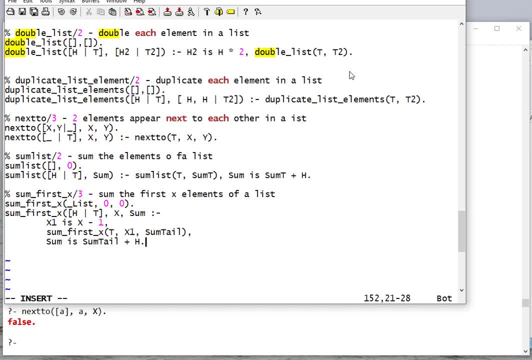 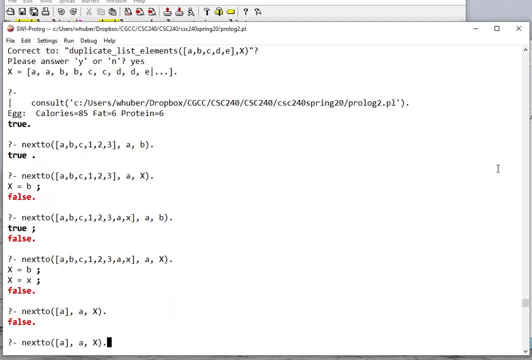 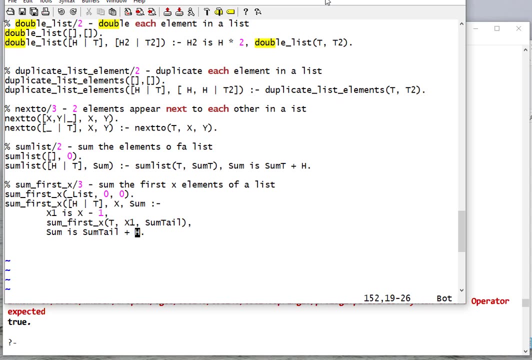 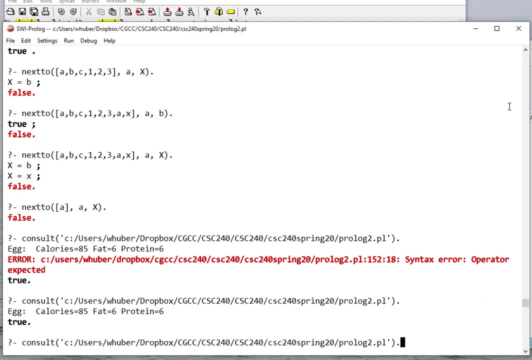 because the first three elements of the list include the first two elements of the tail. Let's test them. So it's saying operator expected. Ah, there we go. So now, if I sum list, it adds those up and you can verify that that's correct. 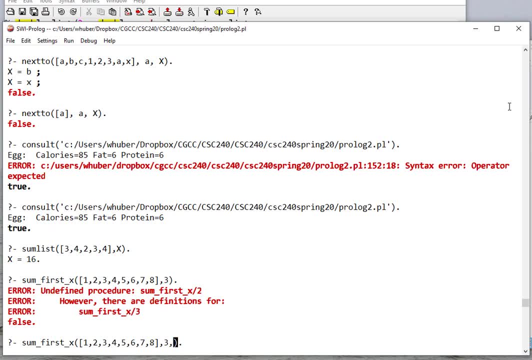 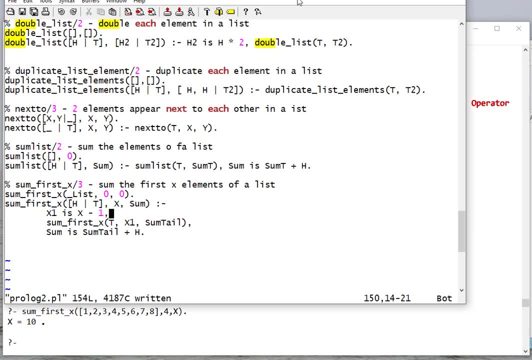 So if I sum the first three, I get six, If I sum the first four, I get 10, and so on. Not every list operation has to be recursive, So I can write a cons rule. It takes an element and a list and returns the pair element list. 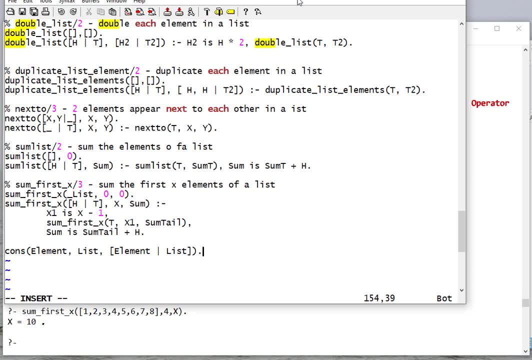 And if that's that actually worked, just like cons and scheme, because if I cons the element with a list, it'll return a list. If list isn't a list, then it's going to be a pair. It'll be a pair anyway, but in that case it wouldn't be a list. 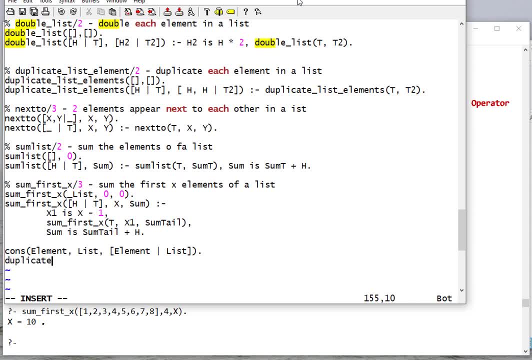 It would be a non-list pair. If I want to duplicate the head and I have head and tail, then I'm just going to unify that with two heads In front of the tail, And both of those rules don't require a lot of logic to them. 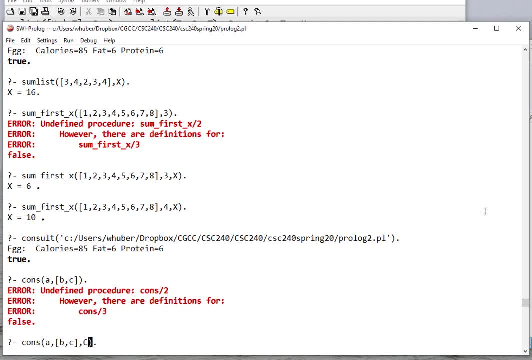 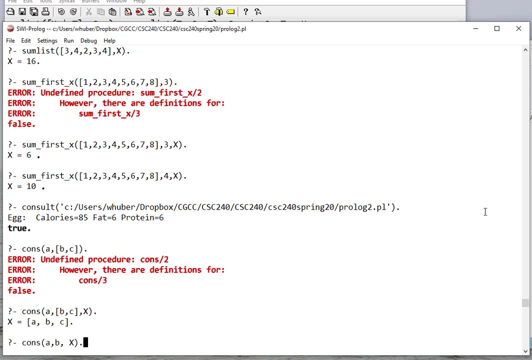 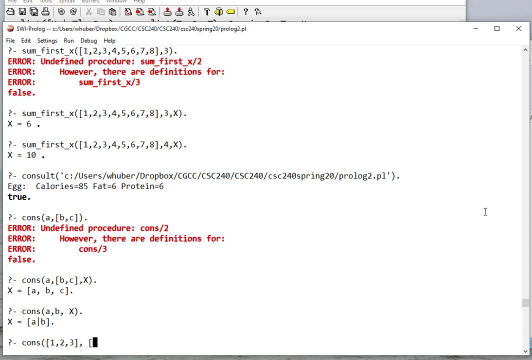 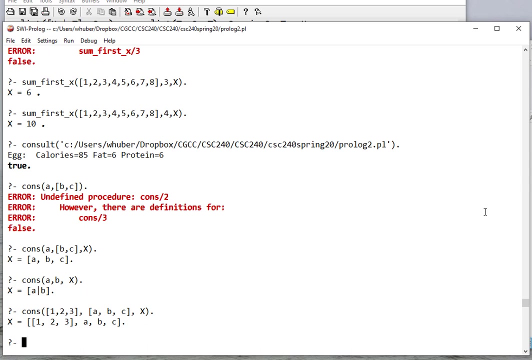 So cons ABC gives me the list ABC, Cons A and B gives me the pair AB. And if I cons the list 1, 2, 3 with the list ABC, there I get the list. 1, 2, 3 is the first element, then A, then B, then C. 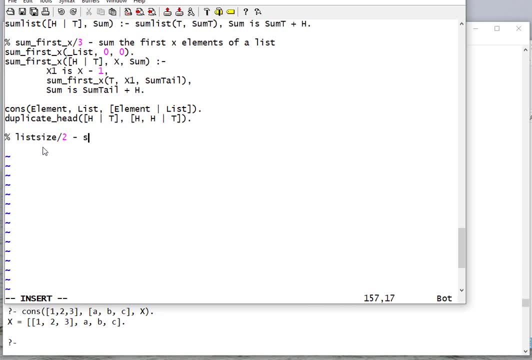 So list size will return the size of the list. Now there's a built-in method that will do this, but we can build this from scratch as well. So the empty list has size 0. Then for a list we don't care about the head. 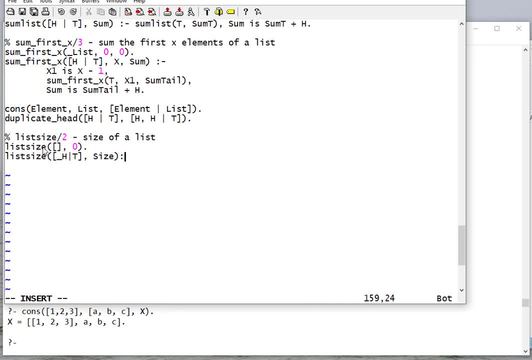 We do care about the tail. The size is going to be the size of the tail, So we're going to add 1 to the list plus 1.. So once we find the list, the size of the tail, then we can add 1 to that. 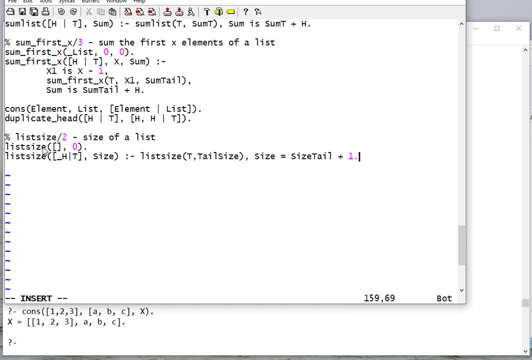 That'll give us the size of the entire list And, of course, as it recurses through this, it'll find the size of the tail. the same way, I can write a rule: add 1 to all. This increments each element in the list. 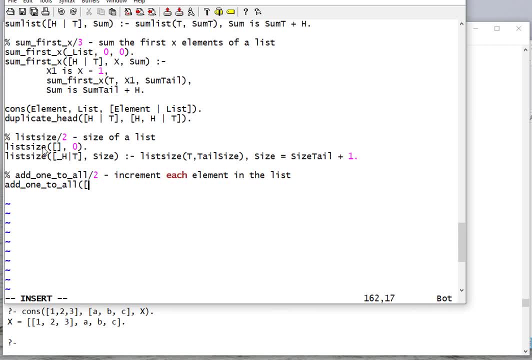 Base case. there the empty list. we're done. So it just could be the empty list. There's nothing to add to. Otherwise, we're going to add 1 to all. So now we have a head and a tail and we're going to add 1 to the head. 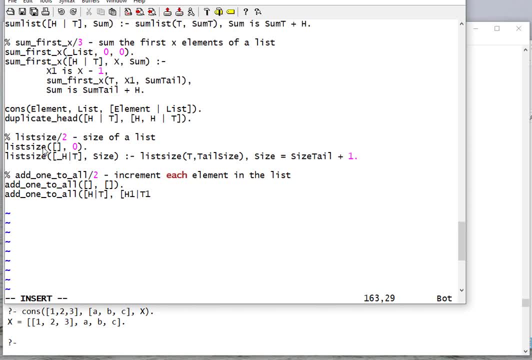 And we're going to increment everything at the tail, So we need to do that in the body of our rule. So h1 is straightforward, It's h plus 1. And then we need to add 1 to everything at the tail. 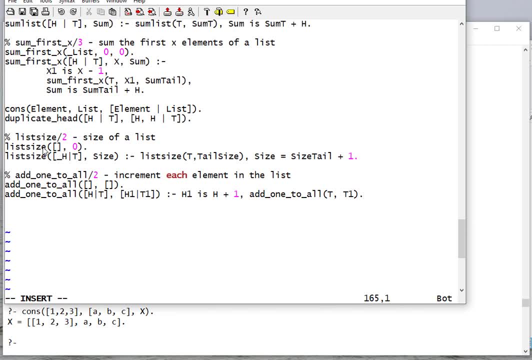 And that gives us t1.. We can also write a more general increment rule Here. We can say: try to use add 1 to all. So if we get a list and to check that we have a list, we're going to only match a list as the first parameter. 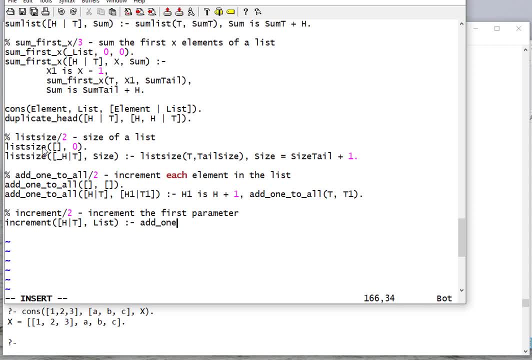 So then this list variable. all we need to do is add 1 to all And now we need to pass the list. But remember, we broke it apart in our parameter, So we need to put it back together here. So this is a complete list. 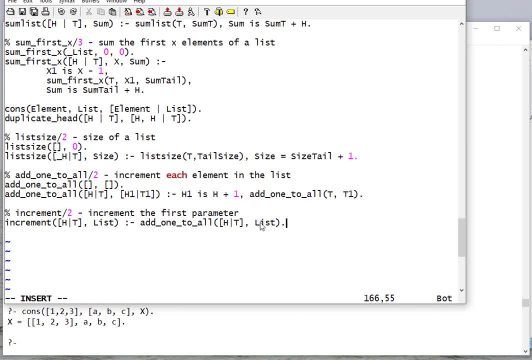 And that's going to give us our result of a list. So we use that previous rule to generate the result here. But what if it's not a list? Well, in that case y is x plus 1. And that's going to be the first variable. 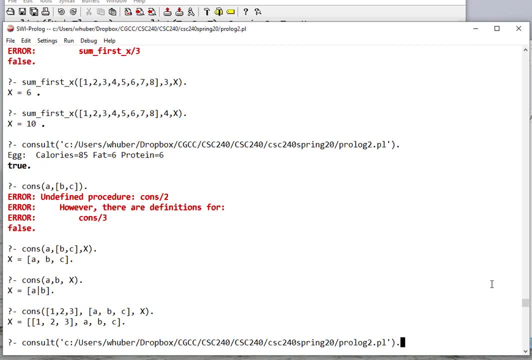 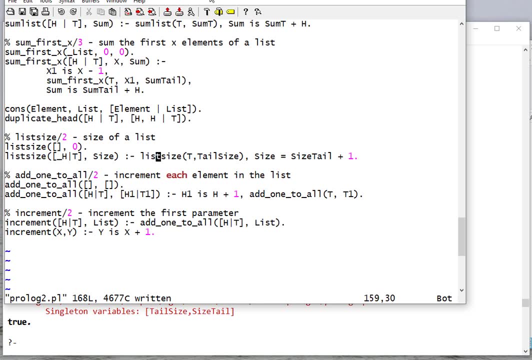 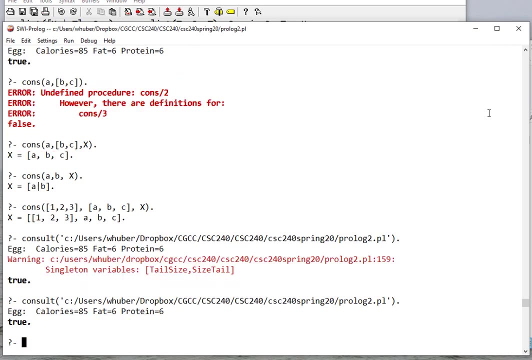 So let's consult. So let's consult. We have a singleton variable. It looks like I reversed my names here, So the list size here and the way that I'm putting it here is going to give us a variable and it's going to give us a number. 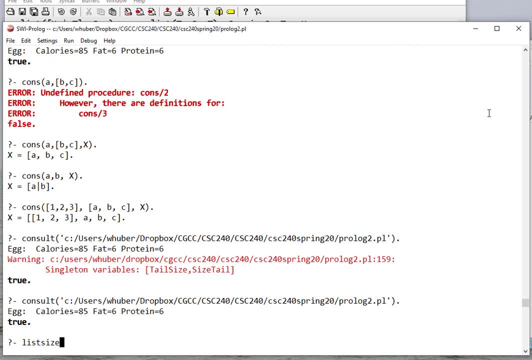 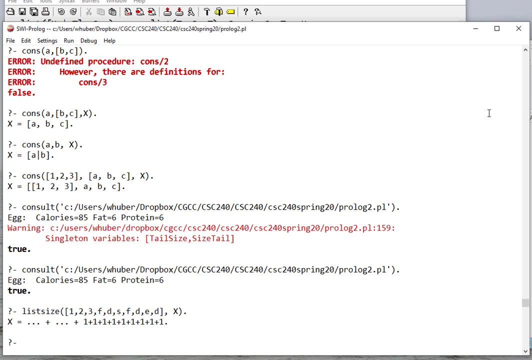 So that's going to be the first variable, And then we need to do the same thing over and over again. So we'll do the same thing over and over again, And then we need to do the same thing over and over again. here is going to be one plus one, so I have something weird with my assignment. oh, I did. 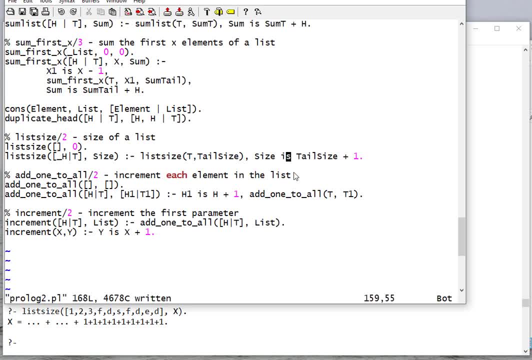 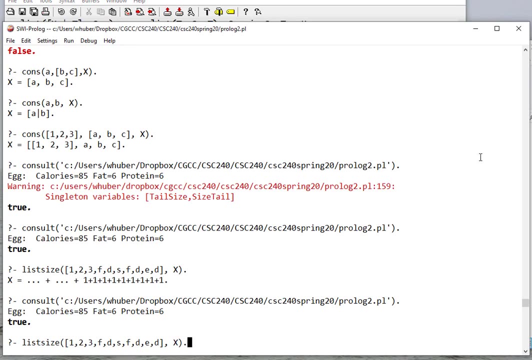 equals. this should be is so that's a good reminder. is is what actually does this operation and then unifies it. if you'll see here, what I did was I had a whole bunch of plus ones. I'm basically saying: unify it with this, with one in the end. so we don't want to do that and that gives me the result I. 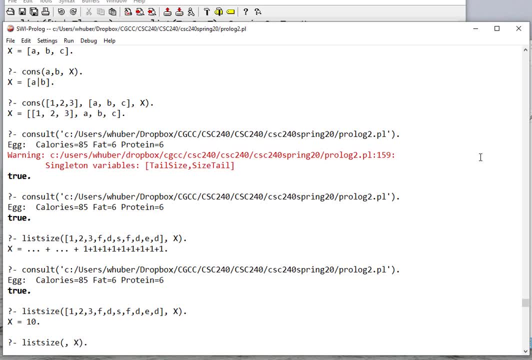 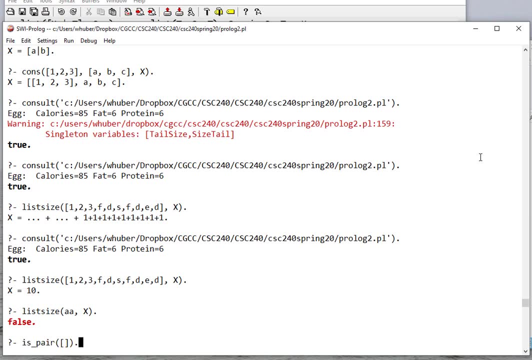 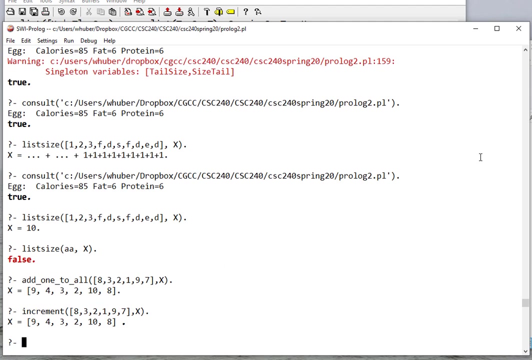 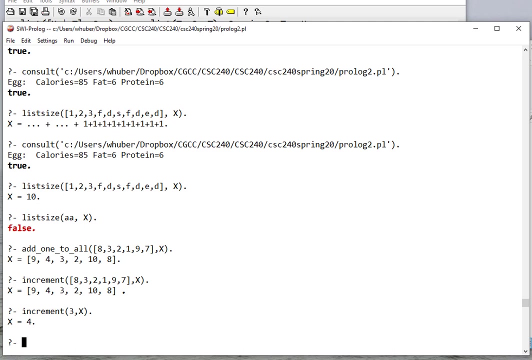 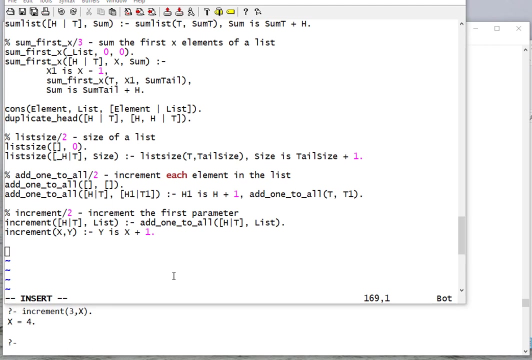 want. if this isn't a list, I get false because that doesn't have a list size. so now I can add one to all. I can also increment that. I could also just increment one of the numbers. so notice that rule works for lists or integers. okay, so let's do a few more. so here's sort of like a filter type rule we're only going to keep. 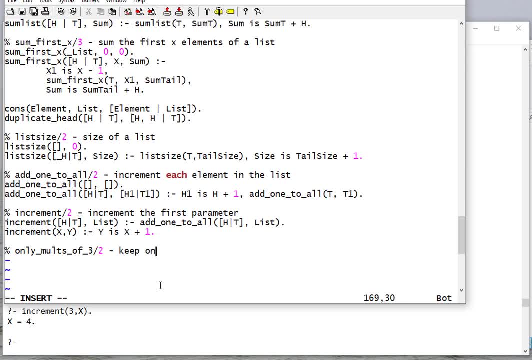 a number here and times. the number you think we have, I'm sorry, is two plus one, and I'm gonna look at option three and I'm gonna push login for the things that we were seeinghosting for the time being. okay, and then, if I'm need the list, I'm just 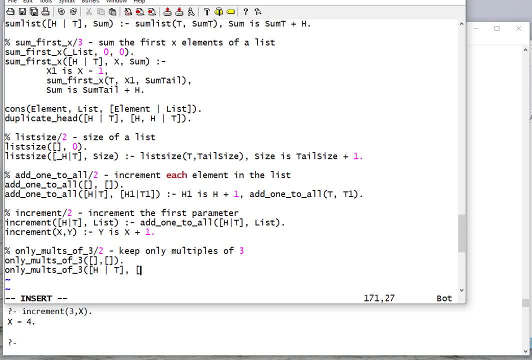 going to set that in. the s4 is supposed to be the empty list. now I'm going to wander around here a And we're going to put the head back on the rest of the list. the recursive result list: only if 3 divides h evenly. 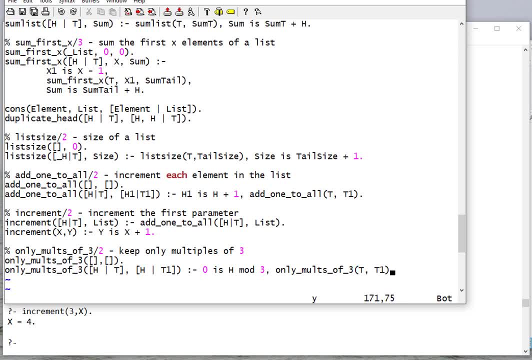 And we're going to get the multiples of 3 from the tail and put that in t1.. Another case would be: if this is not true, So x is h mod 3, and x is greater than 0.. Notice, in this case we don't put the head back on, we just get the multiples of 3 out of the tail. 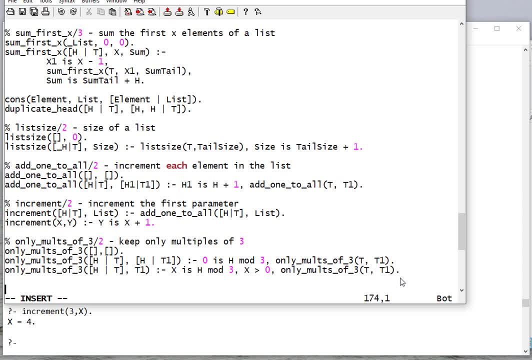 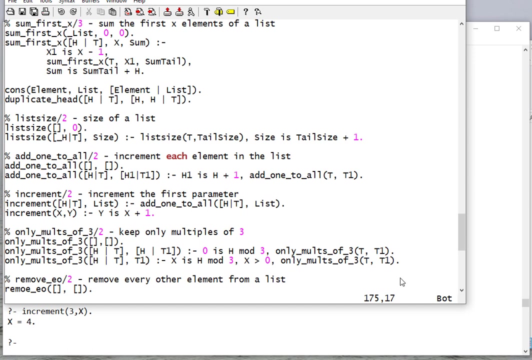 So that's a case where we have multiple conditions and depending on the condition, that determines how we build the result list. Another example similar to that: We're going to remove every other element from the list. So base case. And also, if there's just one element left, then we'll just return the list with that one element in it. 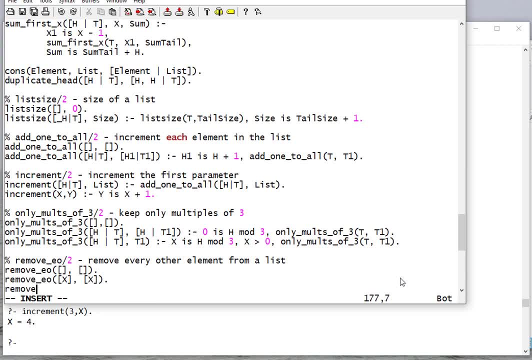 And I need to spell that right- Then if I remove every other element- Now here there's at least two elements in the list, Because I've checked the case where there's one and two. So now there's something on the list and then there's that every other one that I'm going to remove. 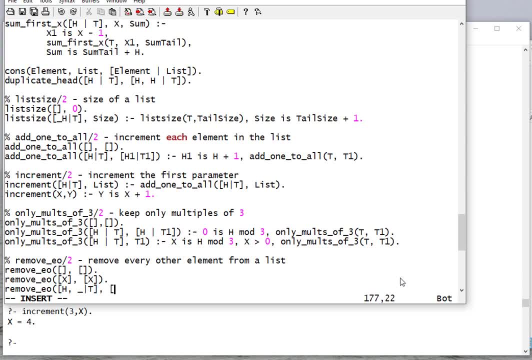 So I don't care about that element And I put the list back on, I put the head back on. The second element I throw away. it's an anonymous variable And then I'm going to do a recursive call on the tail and that'll be the tail of my result. 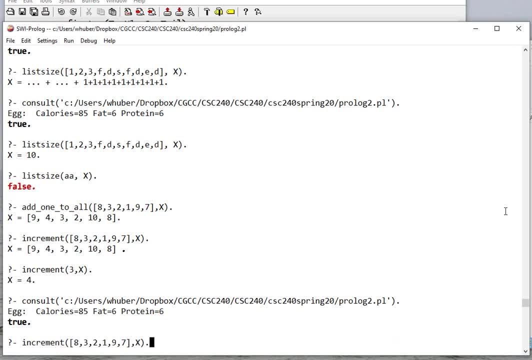 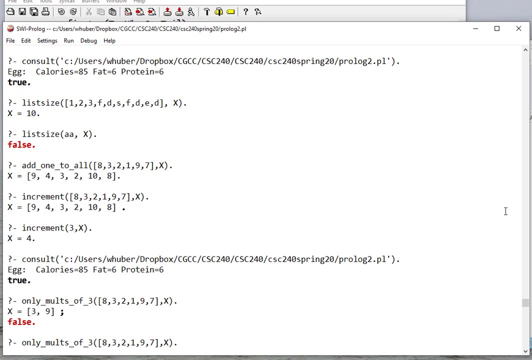 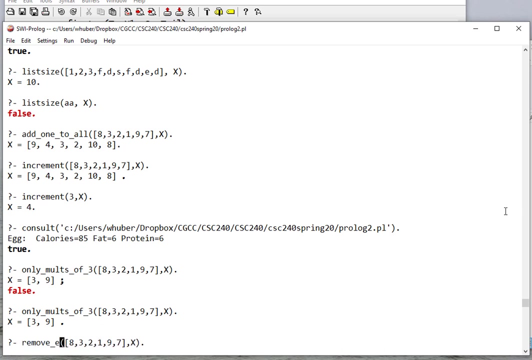 Let's consult, Let's take that list we did before And we'll say only volts of three. That gives me three and nine. It gave me false because I said no, If I just said enter, that would be okay, And then I could also remove every other from that list. and that gives me eight to nine. 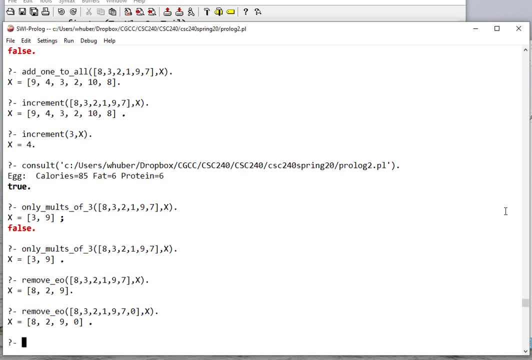 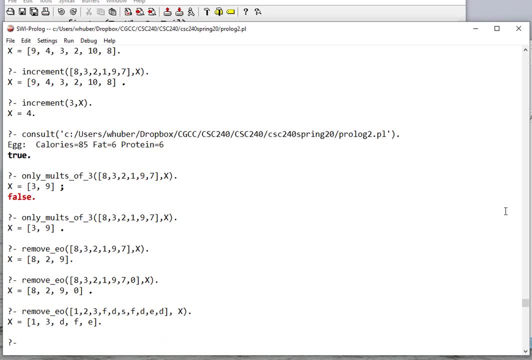 If I had one more element, That would also be there. I think I had a longer list above, Yeah, so let's remove every other one from this one, Okay, so the last example we'll do with this video is: we'll talk about sorting. 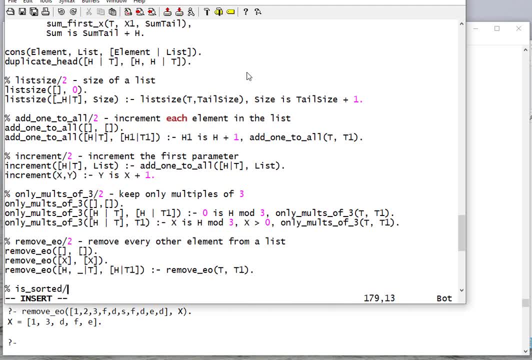 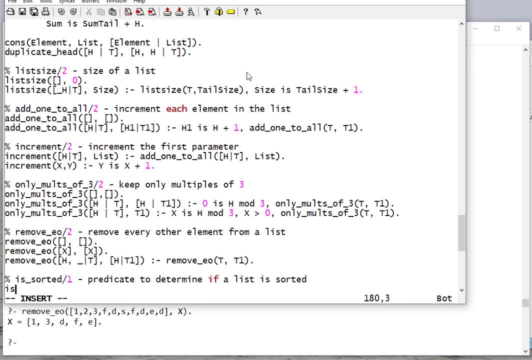 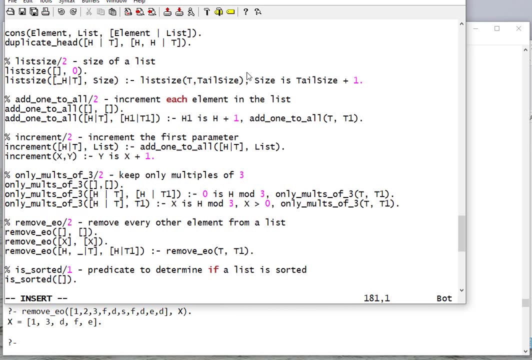 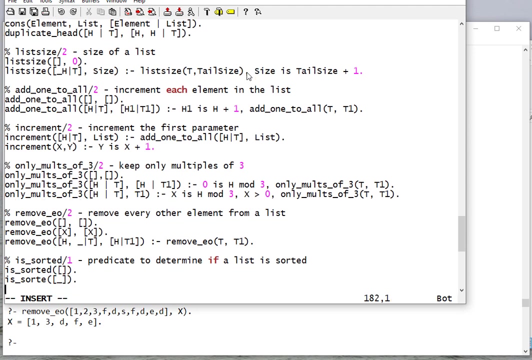 So first off, let's check to see if a list is sorted. So The empty list is trivially sorted. A list with just one thing in it is trivially sorted. So that's an anonymous variable, because I don't really care about it. 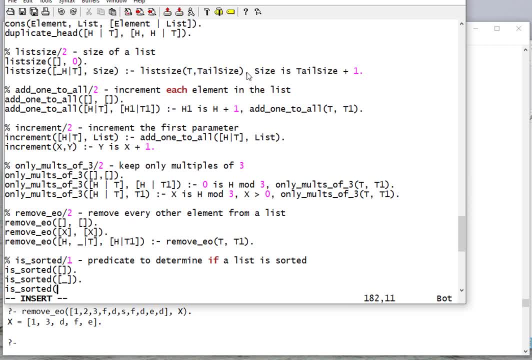 And a list is sorted. if So, here's what we're going to do. First off, the tail is going to have to be sorted. I'm going to have something in the head- We'll come back to that. And the tail. 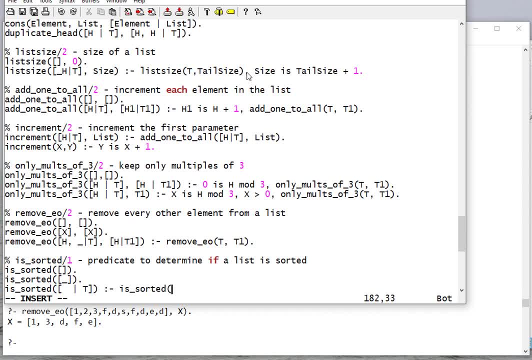 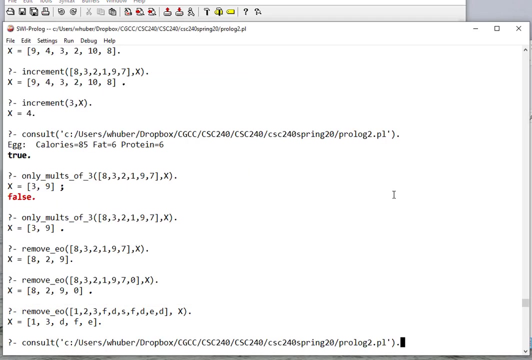 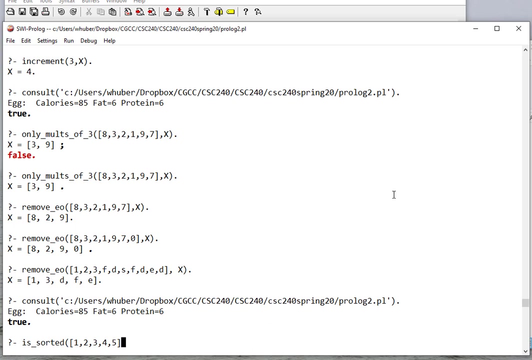 And The tail has to be sorted. So if I say H here, Actually I don't really care about H, right? So let's just, let's just try it like this, Let's see it's sorted, True. 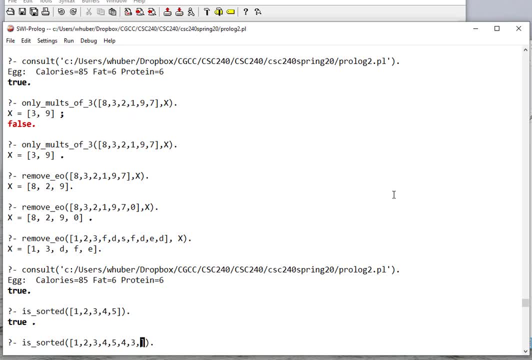 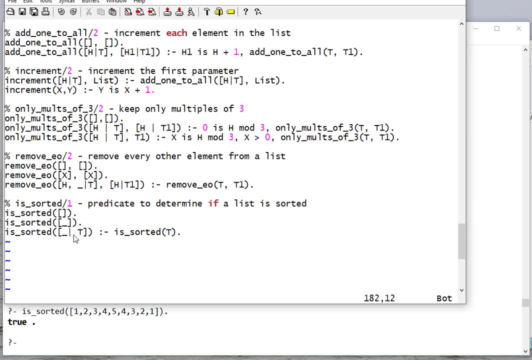 Okay, good. Well, is it good? That's also says true, because what we just basically said is: is this a list With at least one element in it? So, really, what we need to do Is, when you say H one and H two are at the start of the list, 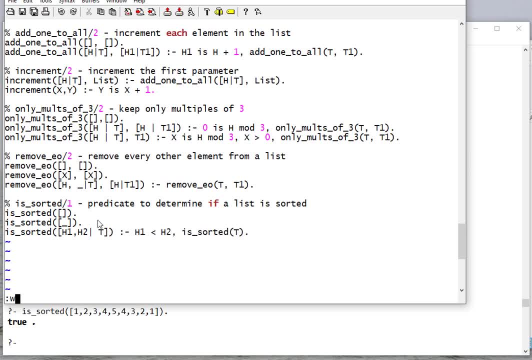 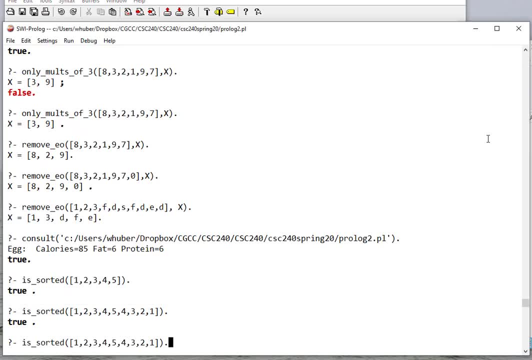 And H one is less than H two, right, Do you see that? Because we need to make sure that the first two elements are in sorted order And then the rest of the list is in sorted order. So let's try that False. 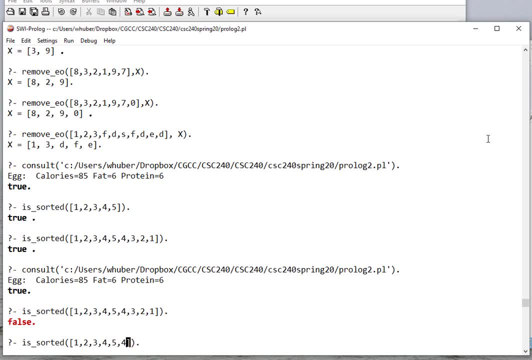 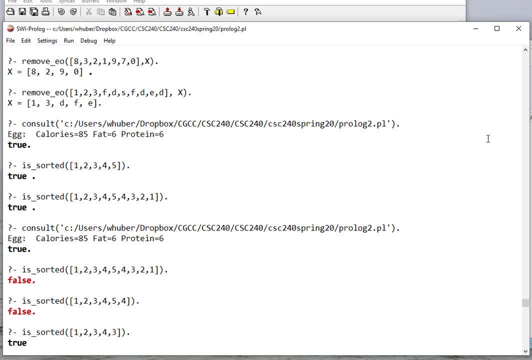 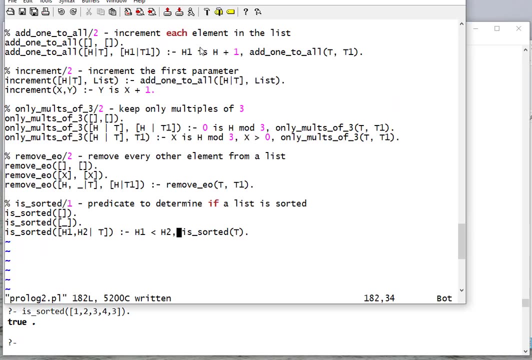 Okay, good, That's what we wanted. That's also not sorted. But that is sorted: One, two, three, four, three. Well, that's clearly not sorted. So why is it saying true? Well, notice here. 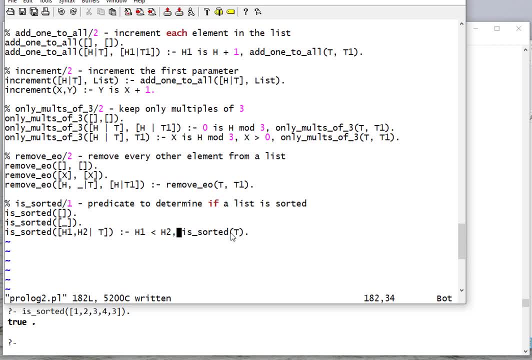 We're saying If these two elements are in order, great, Look to check that the rest of them are in order. But H one is in order but H two might not be. So we want to put H two back on the list that we check to see that sorted with that recursive case. 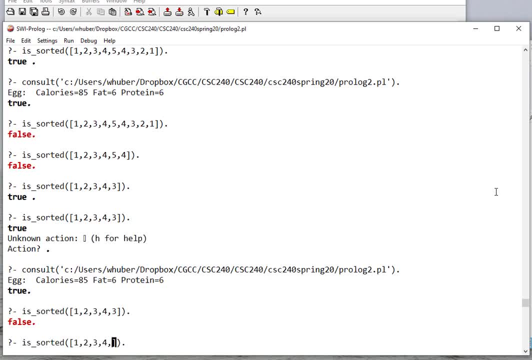 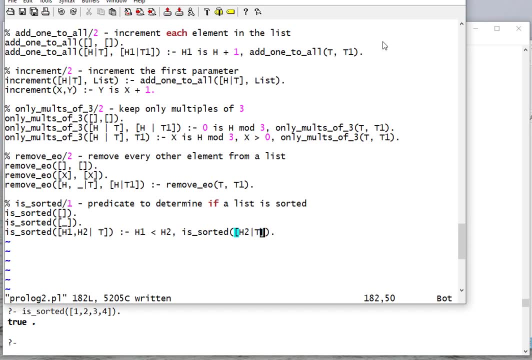 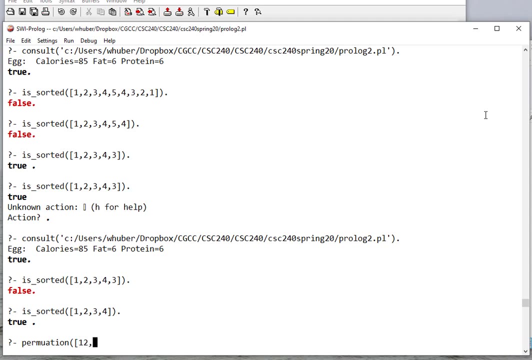 If I consult that, that's not sorted. but that is so now my is sorted rule works the way I would expect. So there's a neat thing in prologue. Say I have a list, one, two or let's say three, four, five, two, one called permutation. 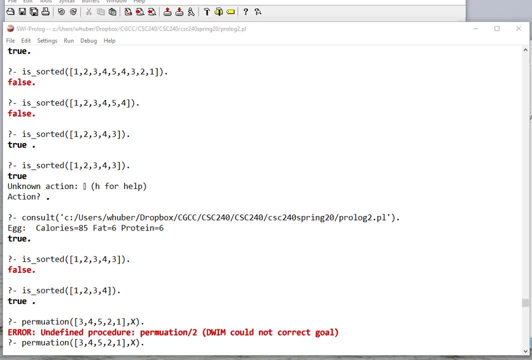 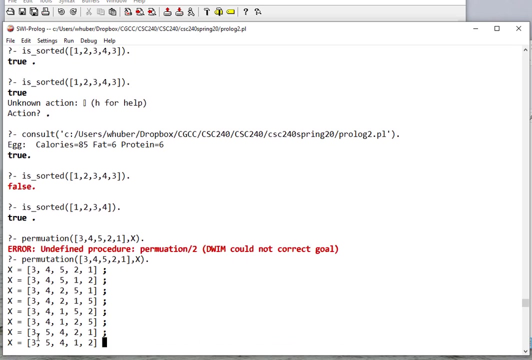 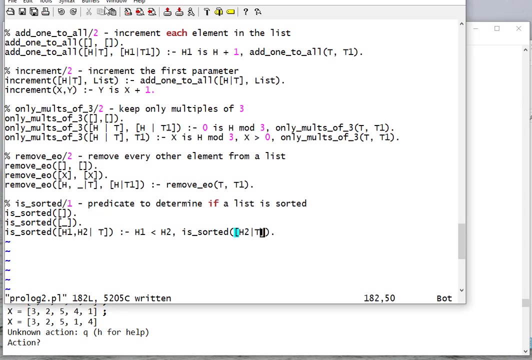 Interesting. I'm going to spell that. there we go. I misspelled it somehow, So notice, if I keep giving this over and over, it'll give me every permutation of the values in that list. Okay, Okay, Okay, Okay. 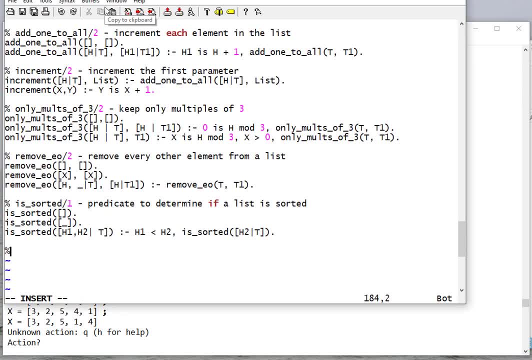 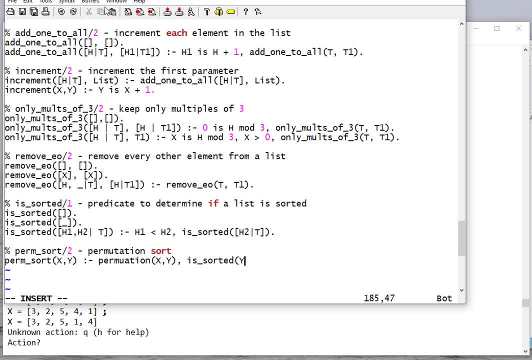 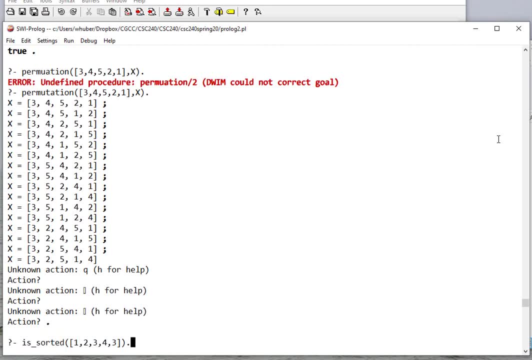 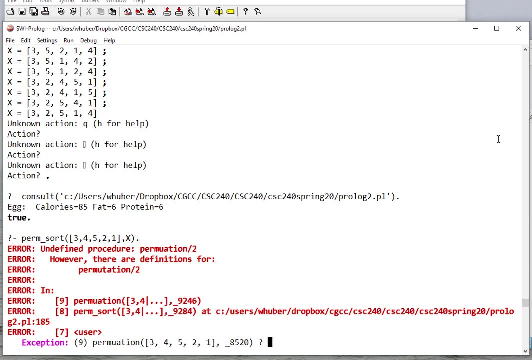 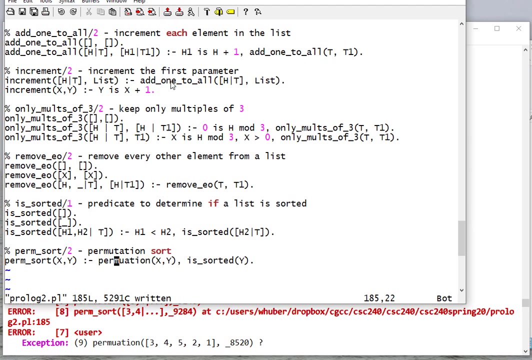 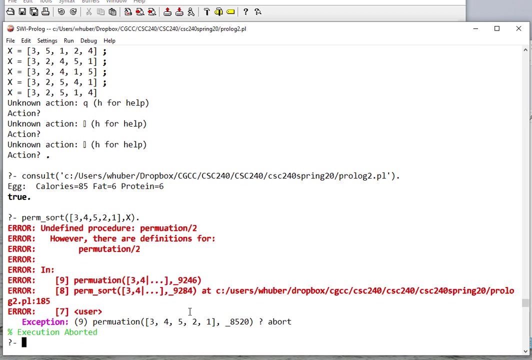 And then I'm going to check: is sorted Y, Okay? Okay, that's my sorting algorithm. So when I consult I can say perm, sort and I misspelled it again. Okay, there we go and notice, it sorts it.